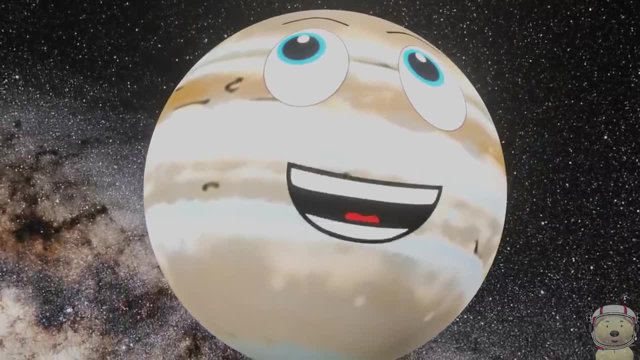 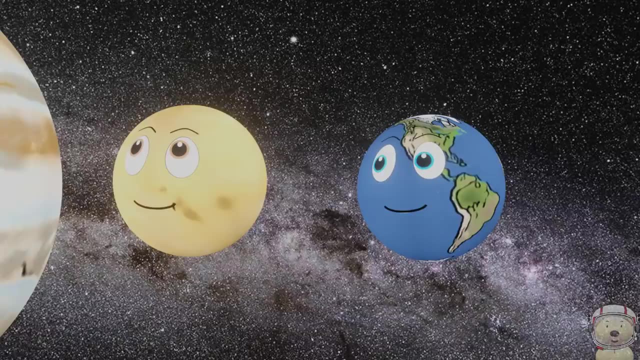 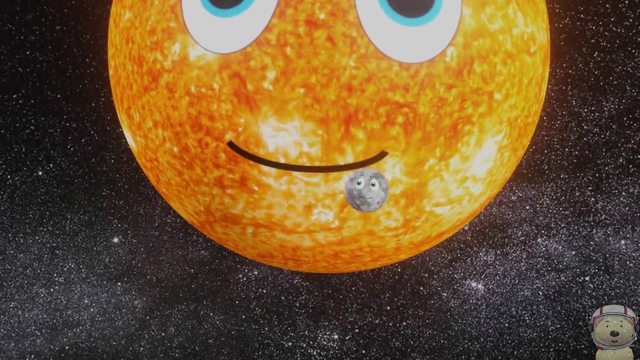 Well, why don't we try it? We can get all the planets together and see if we can do it. I'll go and get Saturn and Mars. you guys get Uranus and Neptune. Wait, what about Wigry? Well, he is so close to the Sun it's hard to get near him without Wigry. 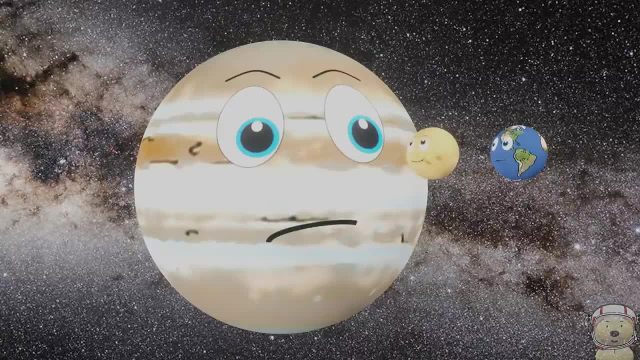 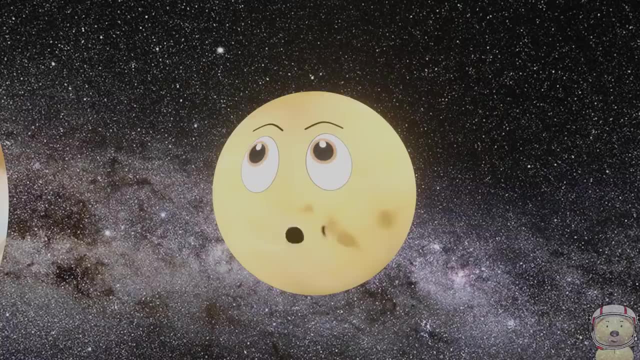 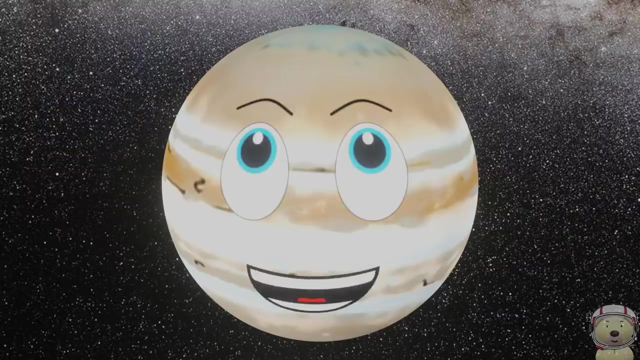 And he's burning up. I'm not sure I want to do it. Yes, very true, And I can't lose all my water. Fine, I'll do it then. Wow, Venus, you're braver than I thought. You're going to risk the fiery heat, That feeling of your very core being on fire as you get closer and closer. 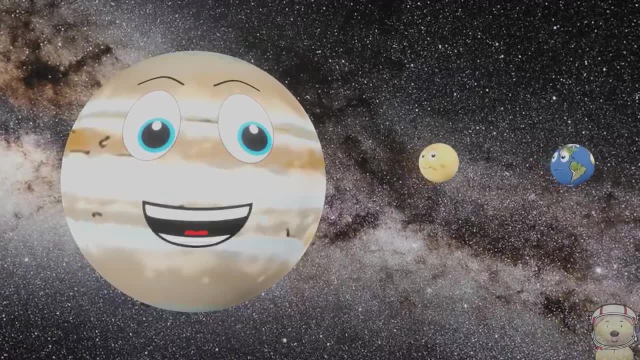 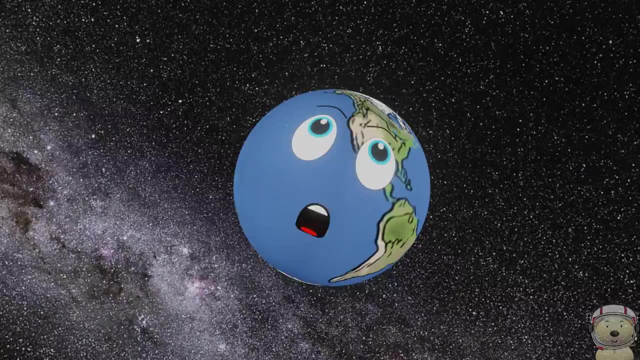 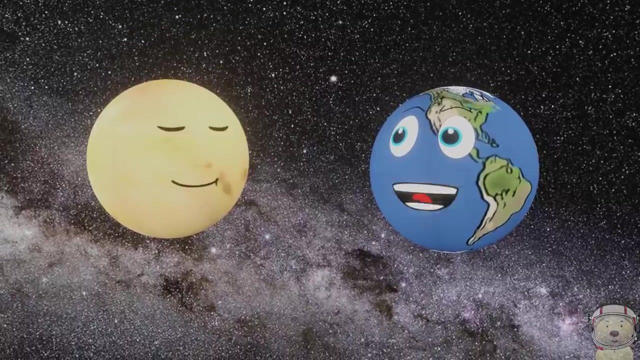 That never-ending burning that will well never, ever end. Yes, those unforgiving sun rays Burning away all your clouds, one at a time, as you approach the centre of our solar system. Oh Venus, that's too risky. 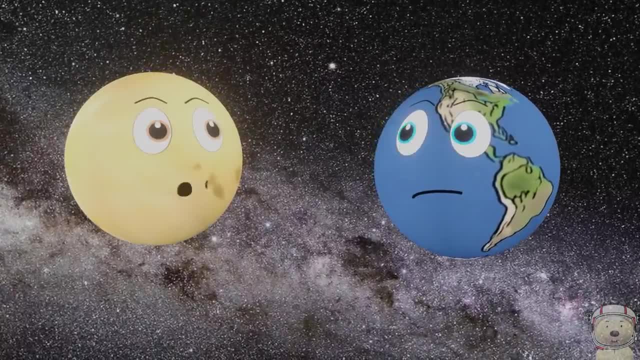 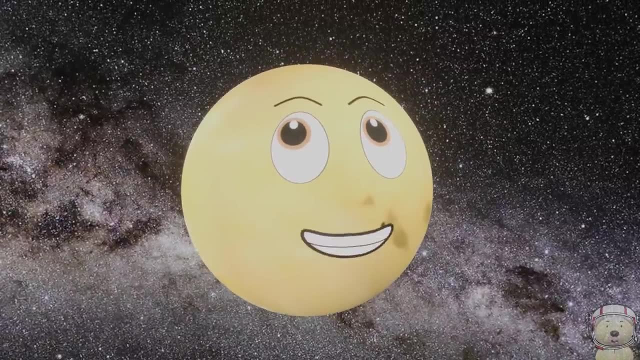 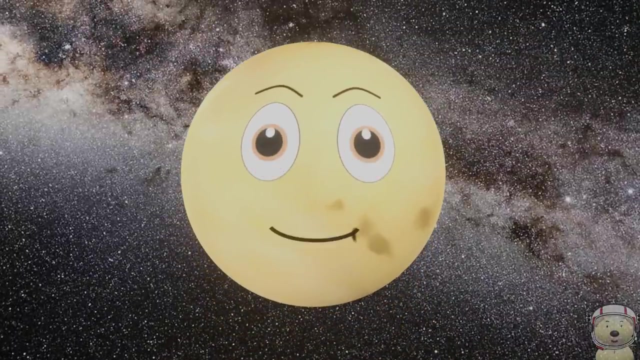 No, I'll, I'll, You'll, what? Okay, I'll miss you. Well, we need Mercury, And I'm the gal for the job. No matter what dangers await, I'll be there. I will face them head on. 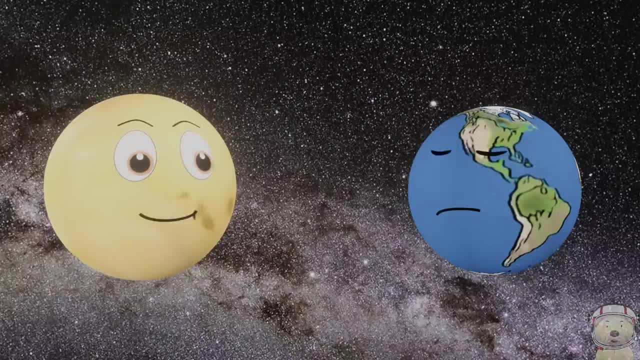 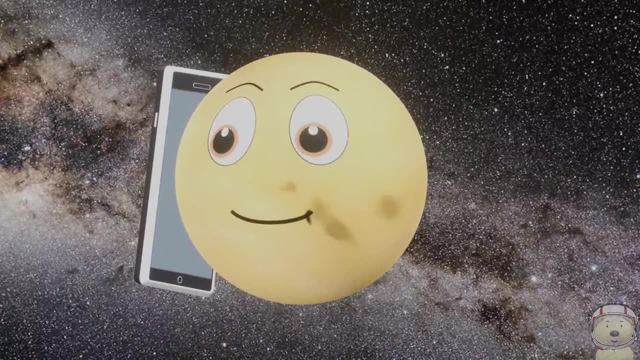 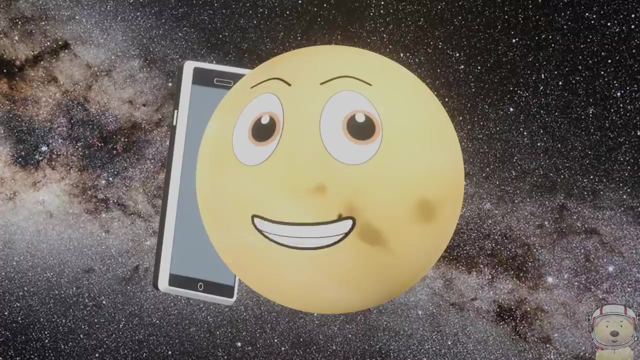 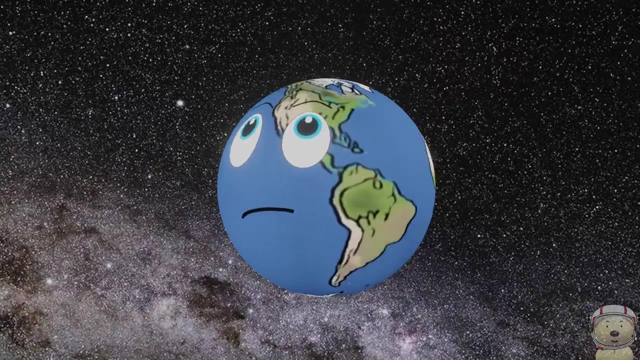 Goodbye, dear friend, Goodbye. I'm just going to call him on his new phone. Hey, Merc, It's we here. Can you meet us near Earth so we can test something out? Yes, Yes, that's right, The small blue planet. 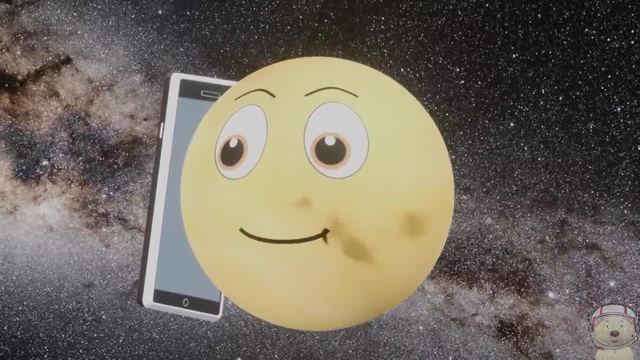 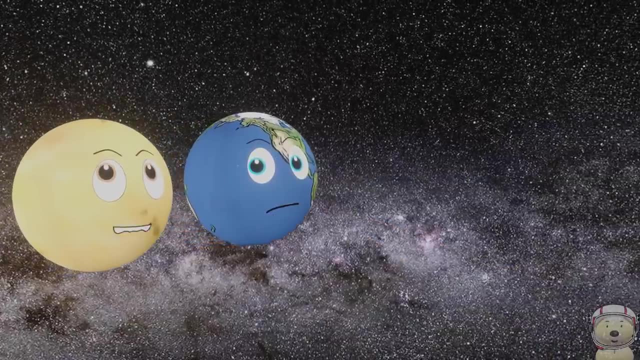 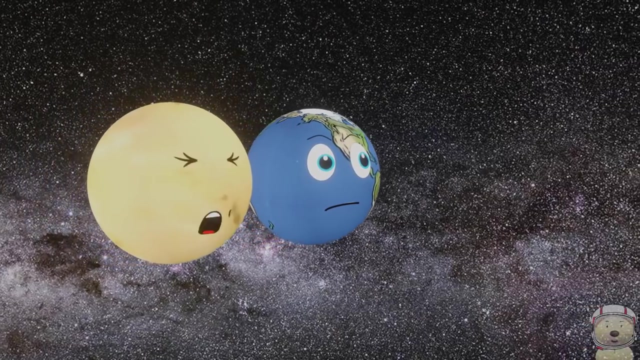 Okay, Send my love to the Sun, Cheerio. What, Oh Venus, I'll miss you more than anything. You're my favourite planet and I love you the most in the Universe. Yes, I never said any of that. 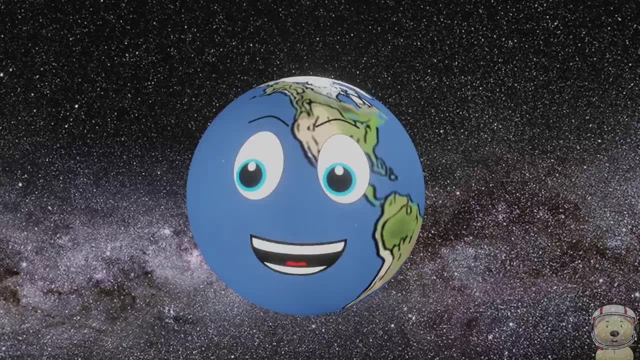 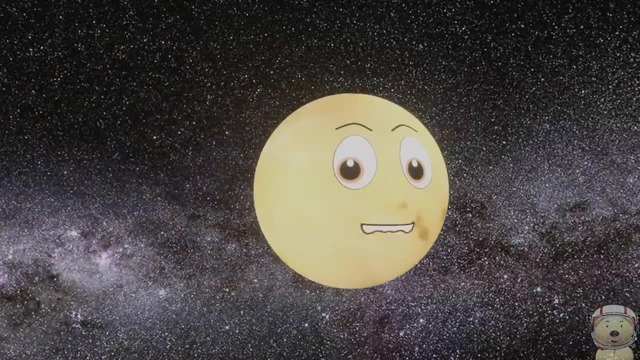 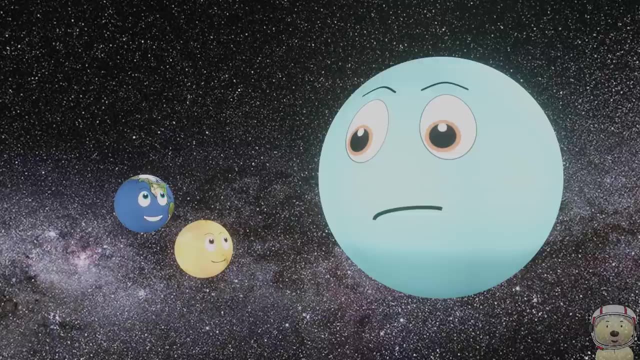 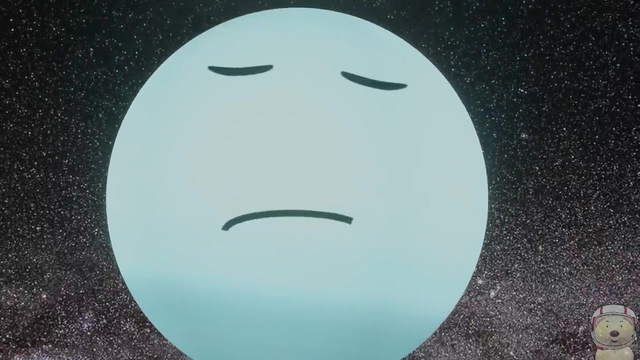 That's what I remember. Well, just remember, I'm bigger than you. Oh, watch out for the asteroid. Hey Uranus, How are you today? I'm very happy today, Are you? Yes, I haven't stopped smiling since I woke up. 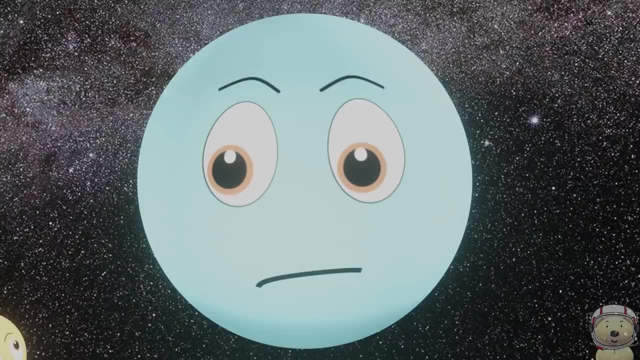 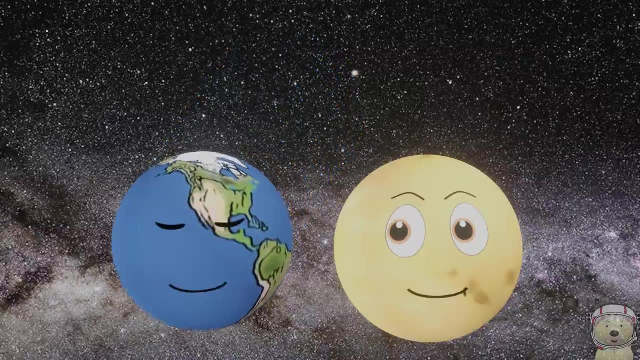 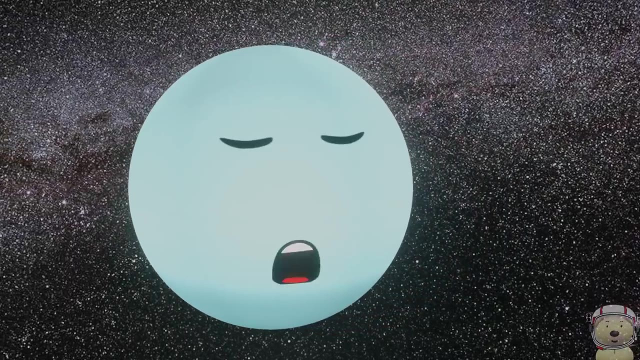 Well, you might want to tell your face. Pardon, I like what you've done with your place. Oh, thank you. Anyway, we were wondering if you could do us a favour, please. You want me to tell you one of my hilarious jokes. 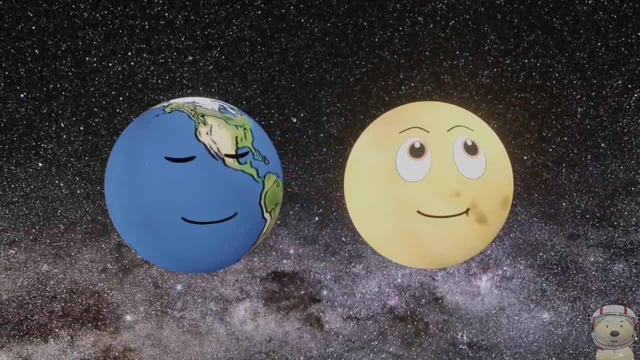 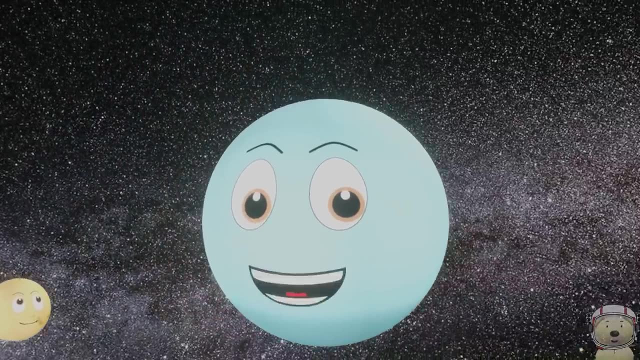 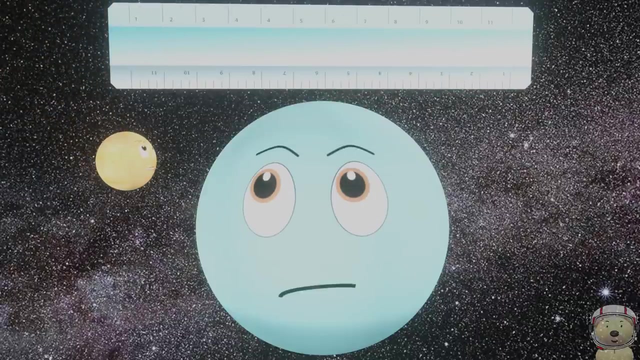 Uh, no, Maybe later We want to do an experiment. How big are you, Uranus? Well, I am over 50,000 kilometres in diameter. Perfect, Can you meet this near Earth's moon please? You can't miss it. It's bigger than Venus. 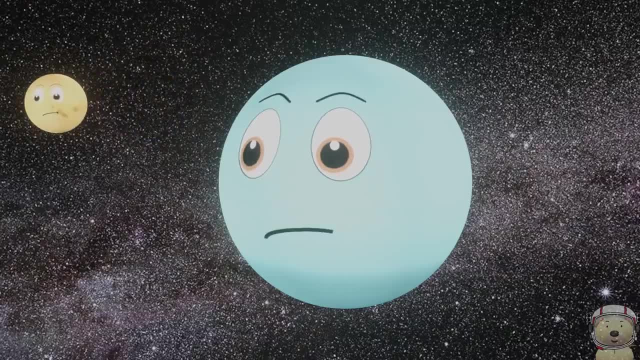 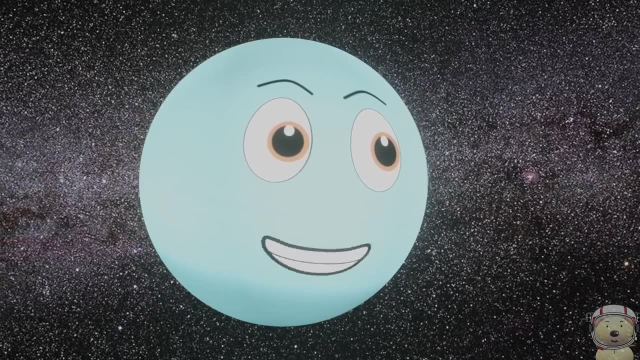 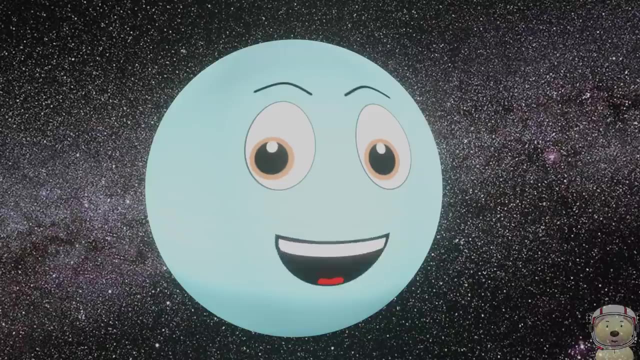 A high five? No, it's not. Well, okay, then I have to go and cheer up some dwarves. I'll cheer up some dwarf planets first, but then I'll be straight over. Does he think he's funny? What did you say? 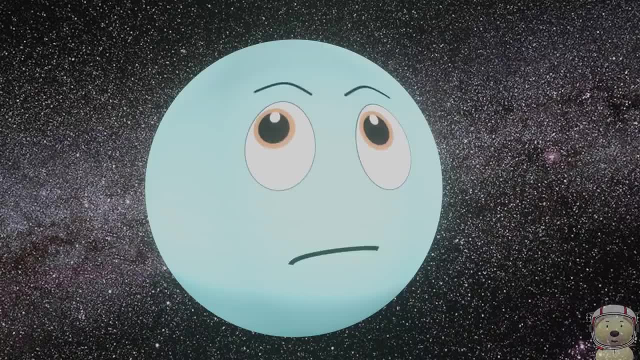 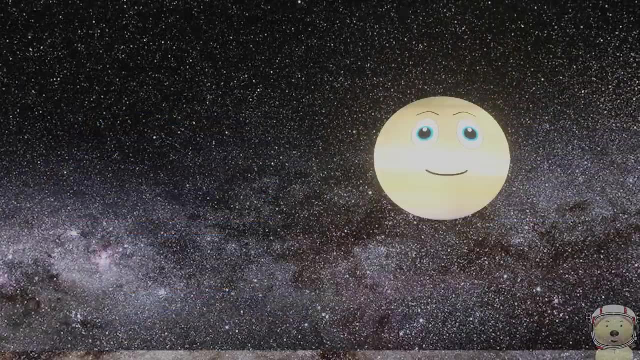 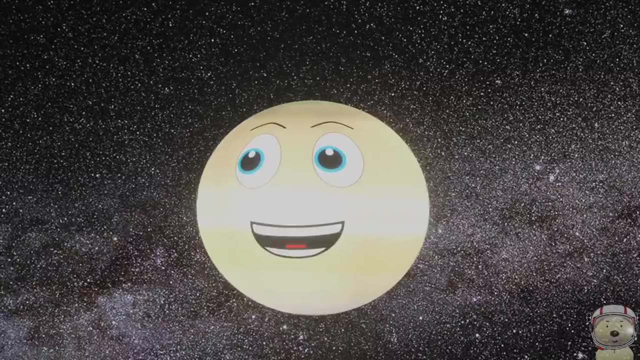 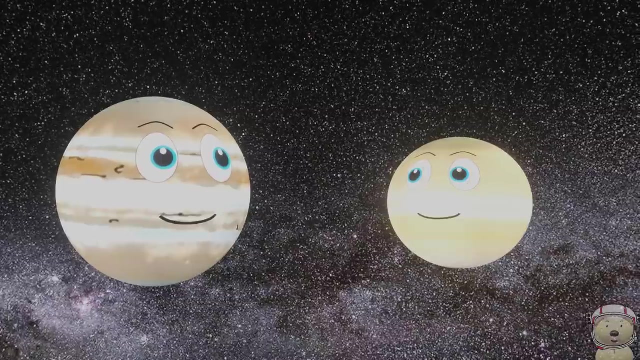 Don't you think it's funny? Well, yes, Yes, it is. How do you do that? so quick Practice SatSaturn, Is it you? Yes, dude, Where's your rings? Just playing catch Catch. 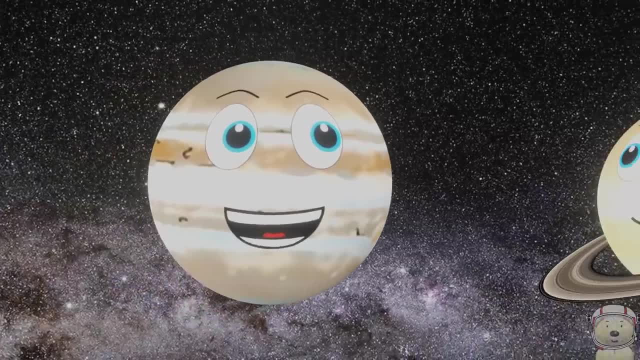 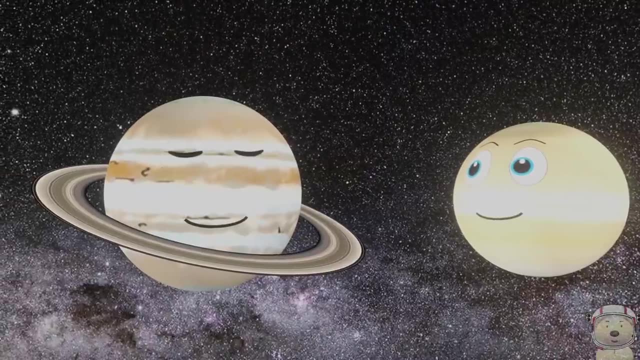 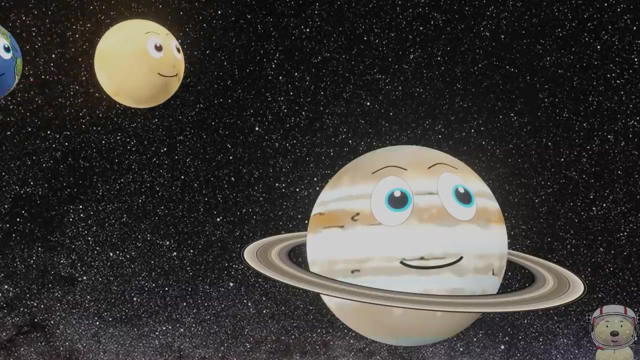 Whoa Neat. I wish I had rings as big as yours. Try it, Alley-oop. Wow, They do look good. They do, dude. They do. Give me another one Earth. What do you say to a rabbit on its birthday? 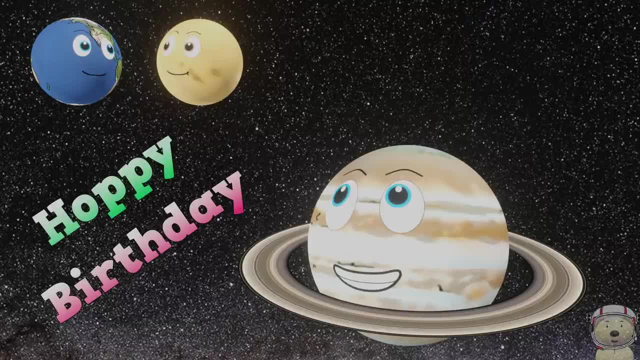 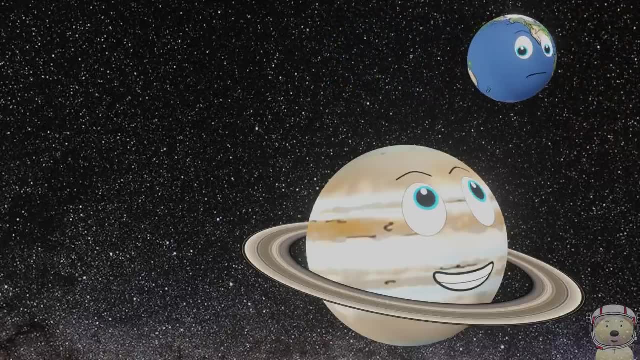 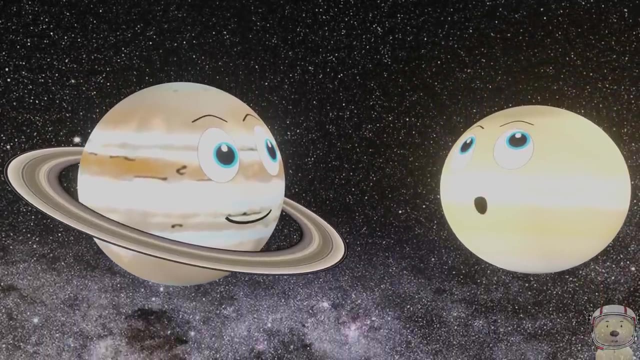 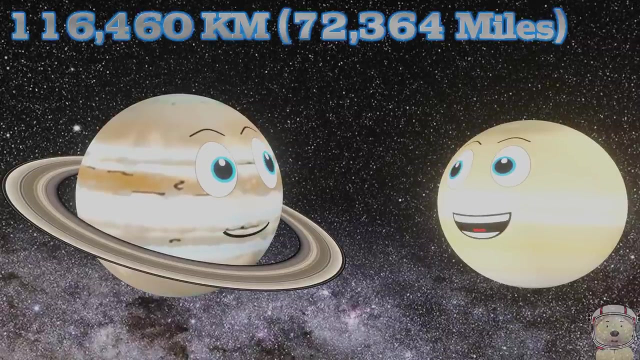 I don't know. Happy birthday, Haha, That is good. Oh, Hey, Saturn. Hey, Sutter, Could you meet us near Earth's moon soon, please, Saturn? Sure, How big are you, Saturn? Well, I am over a hundred and sixteen thousand kilometers in diameter, dude. 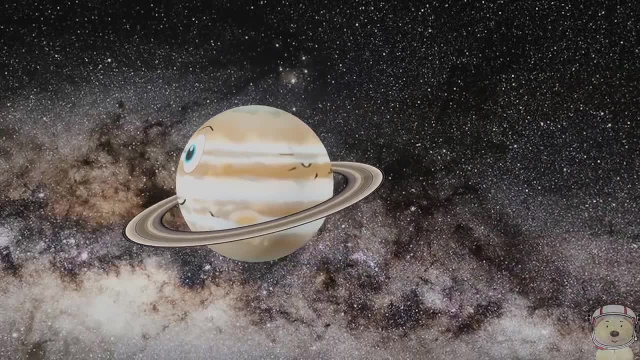 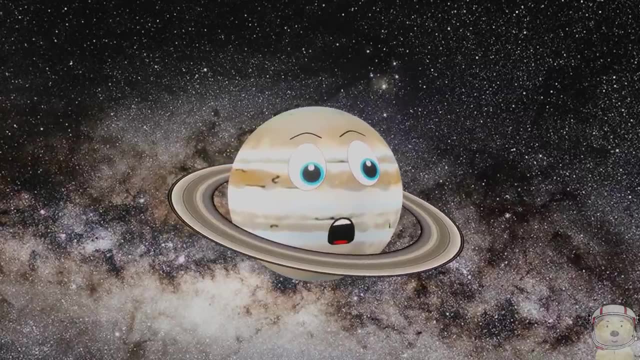 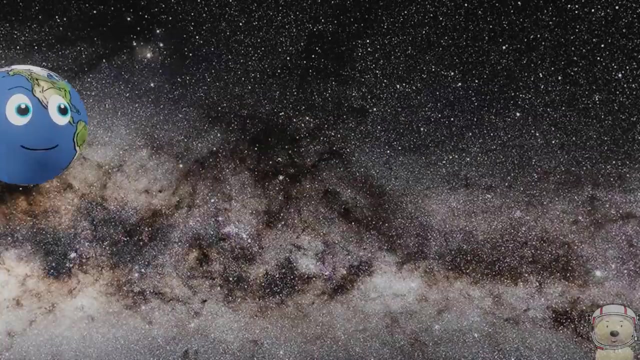 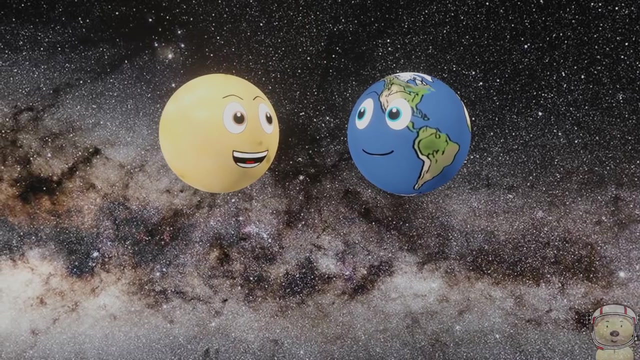 Brilliant. Okay, Catch you later. Hey, Jupiter, dude, Yeah, My rings. Oh, Yes, of course, My bad, I spy with my little eye. Something beginning with S, That's easier Space No, S for small Venus. 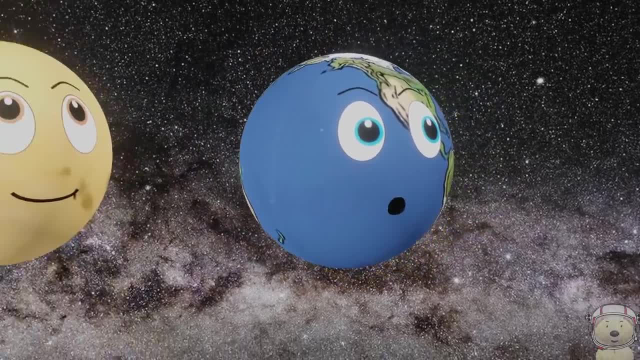 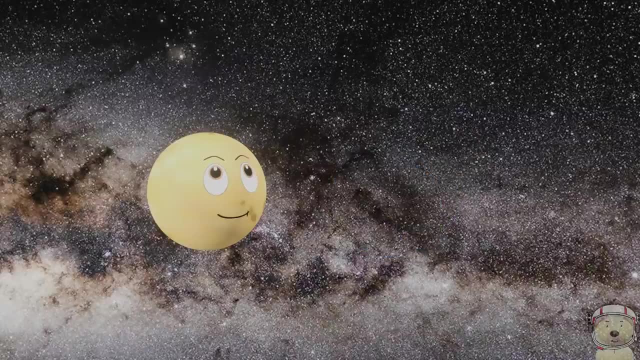 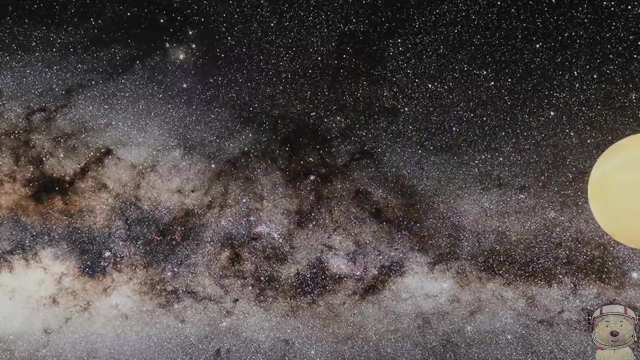 Hahaha, Oh, I am on form today. You'll be on my naughty list soon. Well, you'll be on my Ow. What Did they wake for me or something? Watch out for the asteroid. Wait, Who goes there? 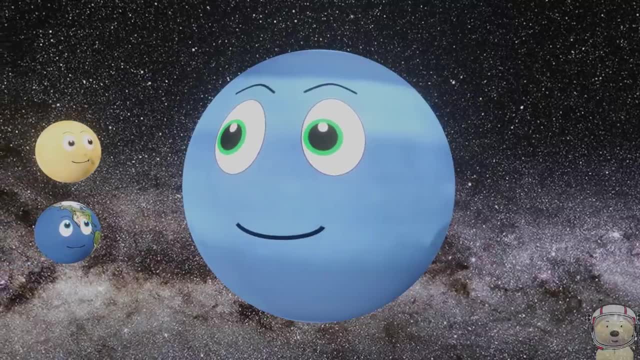 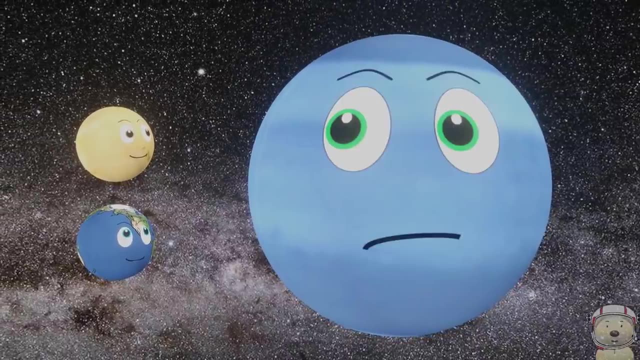 Hey, Neptune, It's only us. Yeah, Calm down. What's wrong? Well, Uranus has been over here again trying to tell me more of his jokes. Are they funny? They are not Being the windiest planet in the solar system. 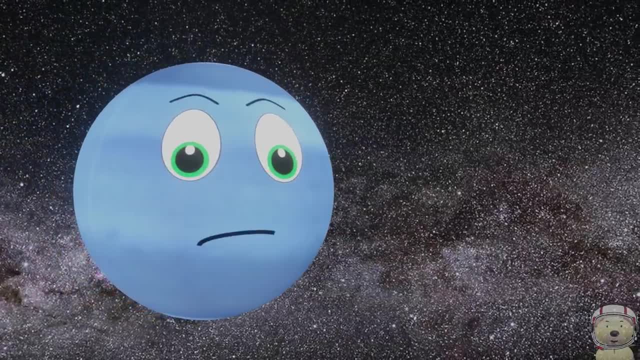 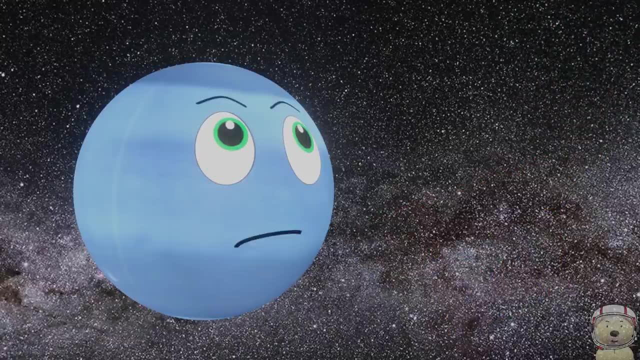 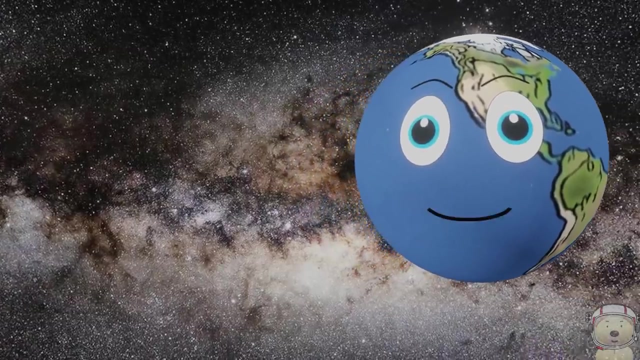 he tried telling me that my favorite day of the week was a Wednesday. Ha, A Wednesday, Brilliant Uranus. no See, He makes me so cross with him. Never mind, It will all blow over soon, Hahaha. 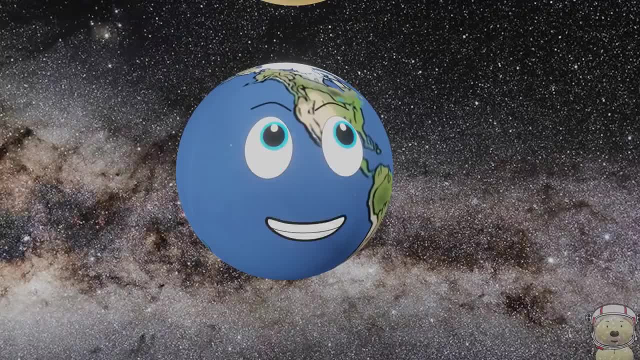 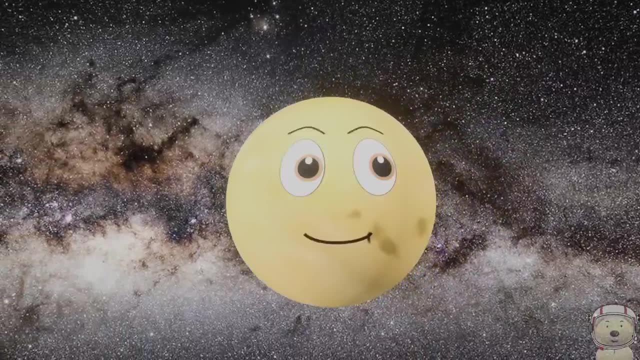 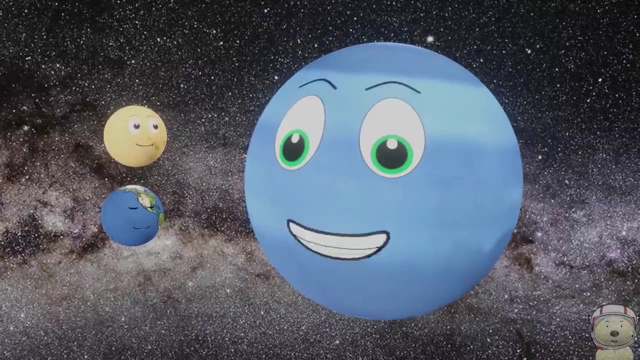 B-blow because of the wind. Do you want me to be cross with you too? Leave it pal. Anyway, NEP, We were wondering if you can meet us near Earth's moon. We're trying out an experiment. Ooh, Sounds exciting. 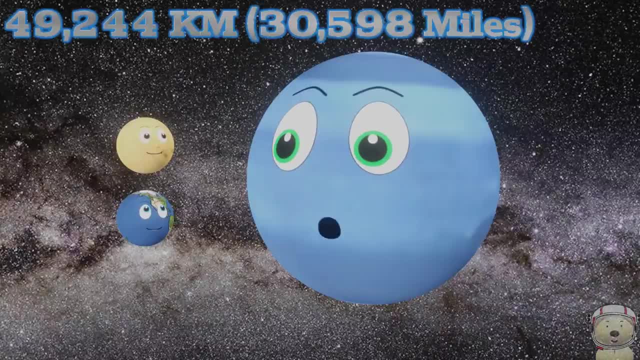 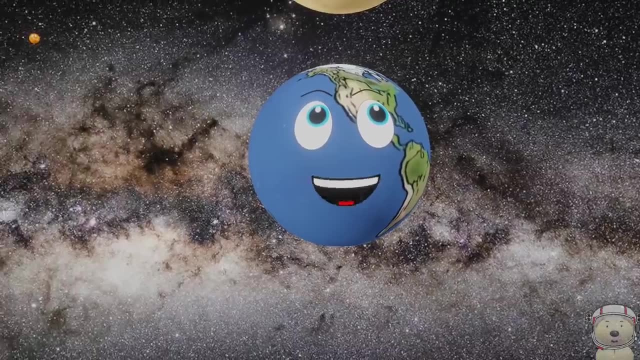 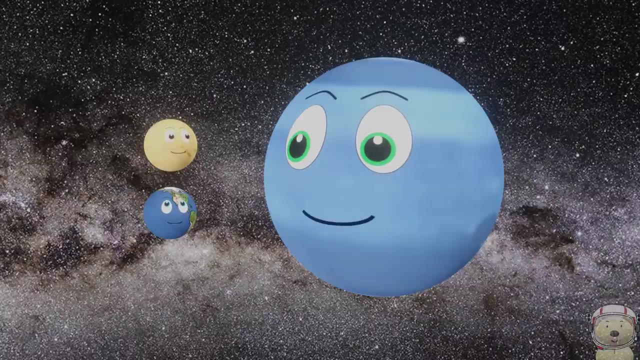 How big are you, Neptune? I am nearly 50,000 kilometers in diameter, Excellent, Um, we need to get back quickly And we are near the end of the solar system. Can you help us out, please, Neptune, Sure, Get ready. 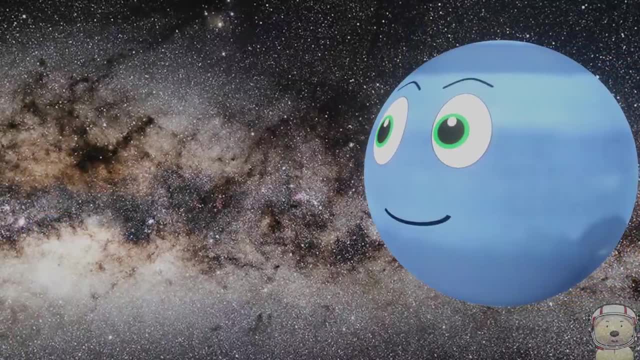 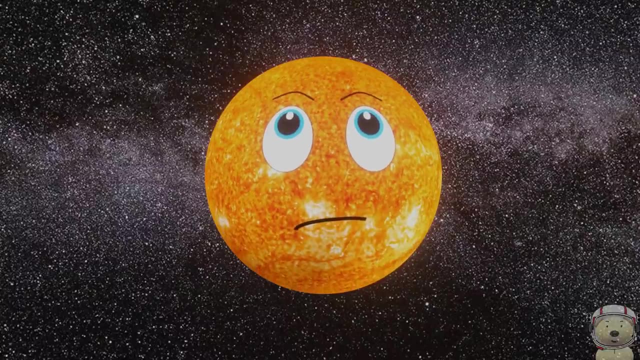 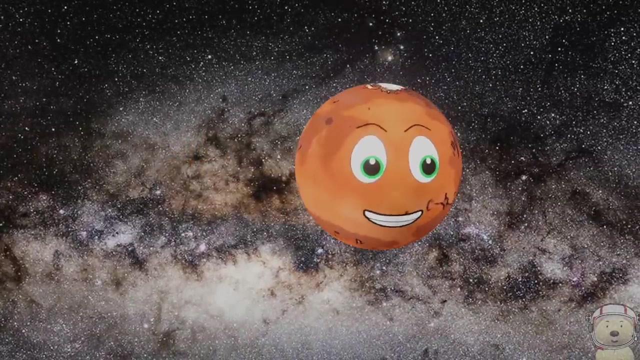 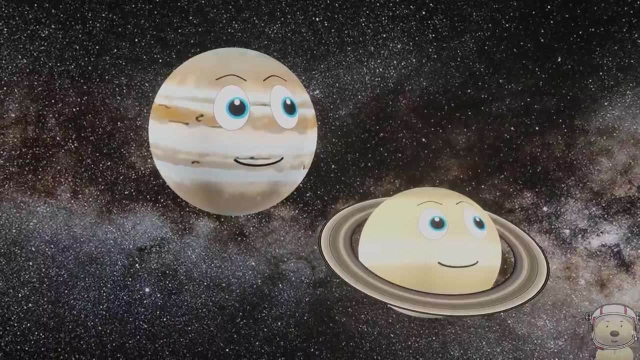 Ugh, Thank you. Woohoo, Woohoo, Uh. My name is Mars, I'm rocky and I'm red. My surface is dusty, stiff. Oh yo, Jupiter, yo Saturn, how are you? That's some good rapping, Mars. 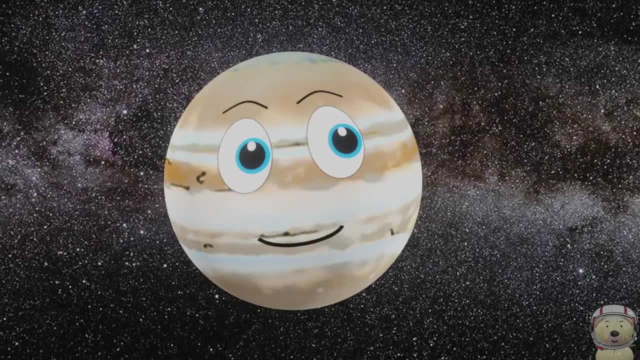 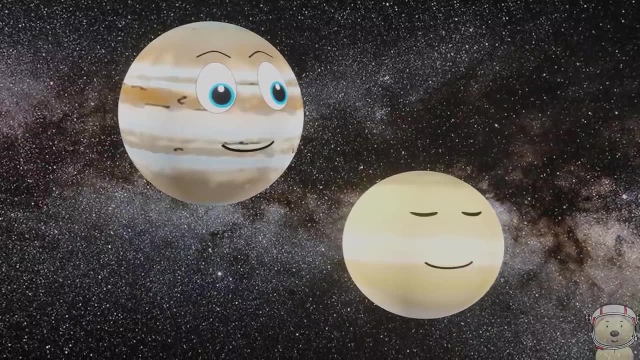 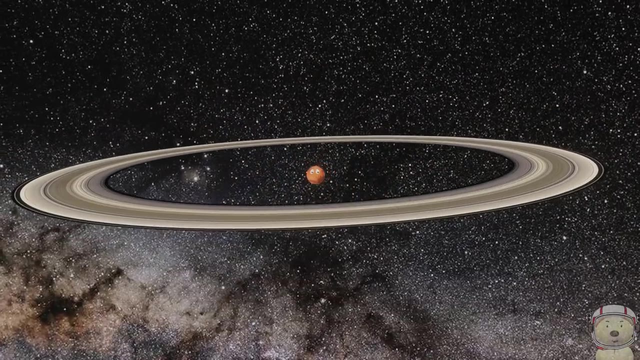 Who are you rapping for Me? Oh, anyway, do you mind coming with us to help us out? What? Hey Mars dude, you look cool with my rings. on What rings? Oh, yes, I'll help out. 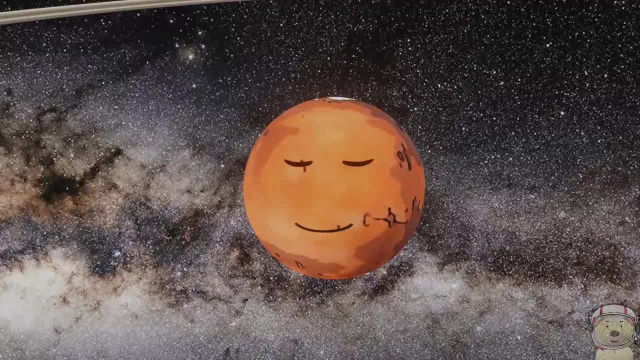 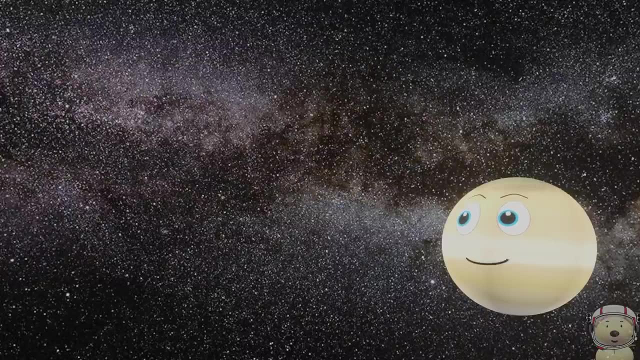 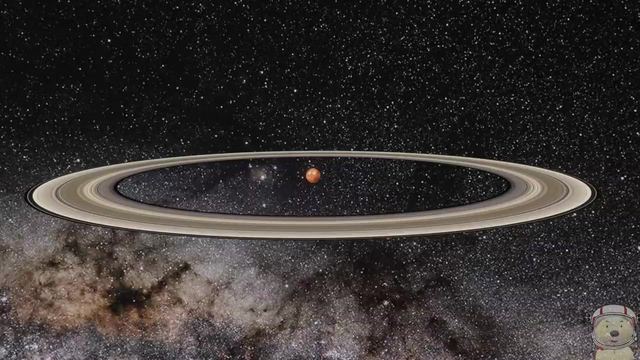 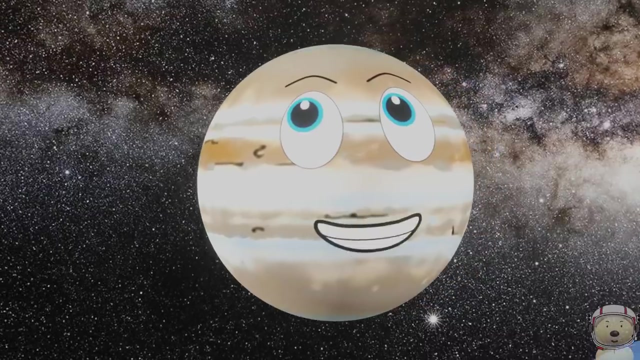 How big are you, Mars dude? Well, I'm over 6,700 kilometres in diameter. Come on then, Mars. Yes, come on, Mars dude. bring my rings with you please. Ah, Ah, Okay, okay, guys, welcome. 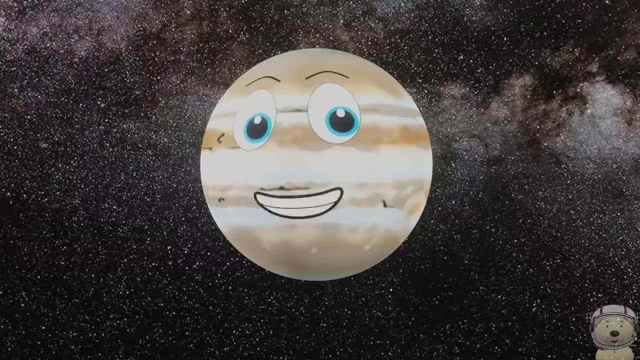 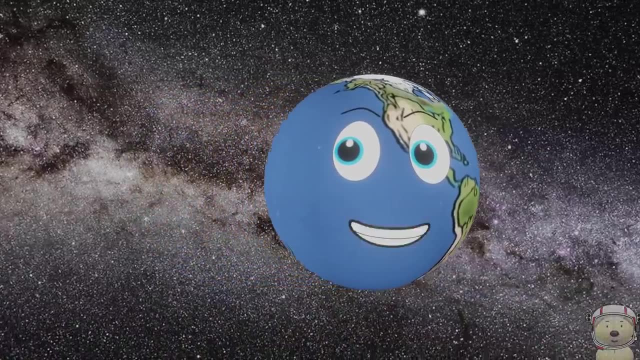 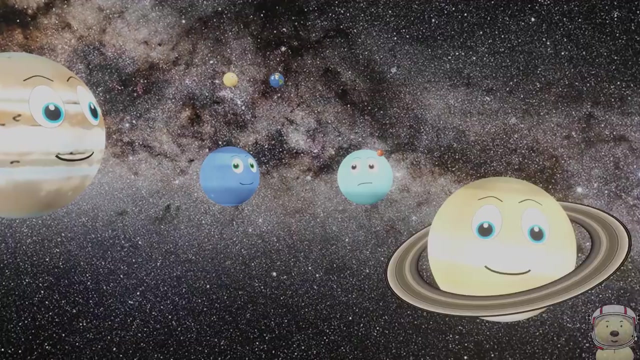 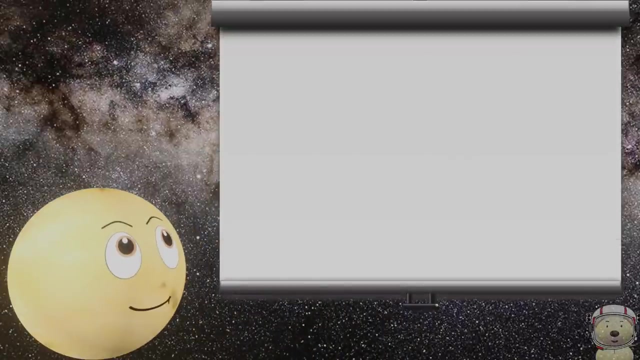 Why are we here? I'm glad you asked my windy friend, That's me. Ah, We were told that you could fit all of you planets between the average distance between me and my moon. Wow, What, Uh, Venus? See here's Earth and here's the moon. 384,000 kilometres away, three circles are our skies. 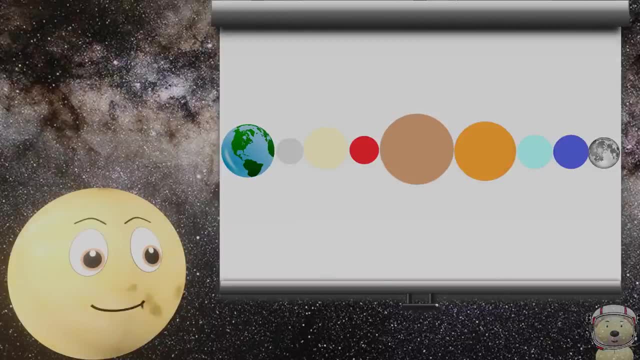 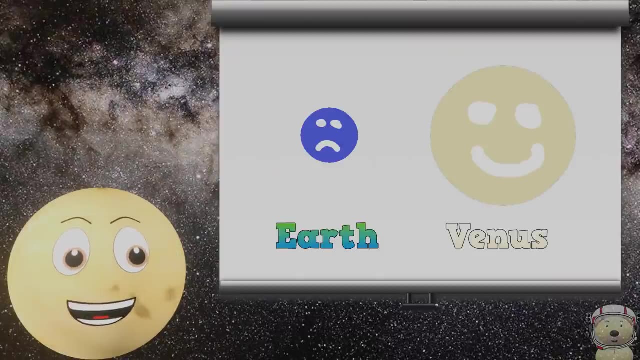 We've got to line up and see if it's true. Thank you, Venus. And this is a diagram of Earth and I Look the big difference in size. Venus, we're about the same size. Why do I bother? Anyway, I'm going to have to go. 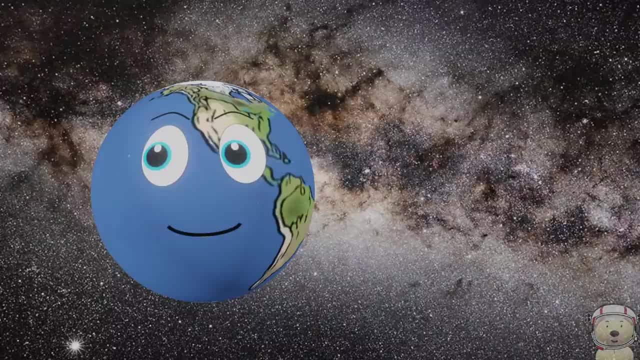 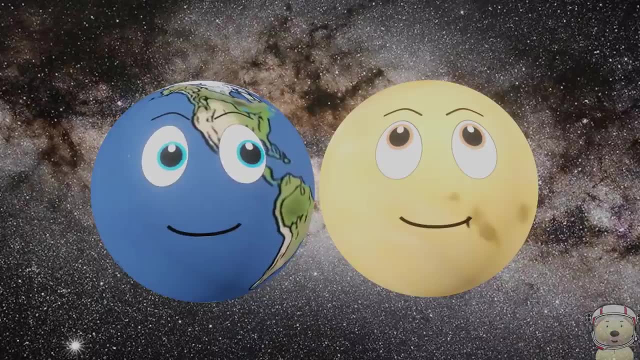 I'm going to have to go, Anyway, shall we start? Okay, first in Venus, Same size Mars, in you go, Here we go. Mercury, Woohoo. Next up Neptune, Hey guys. Next up planet Uranus.